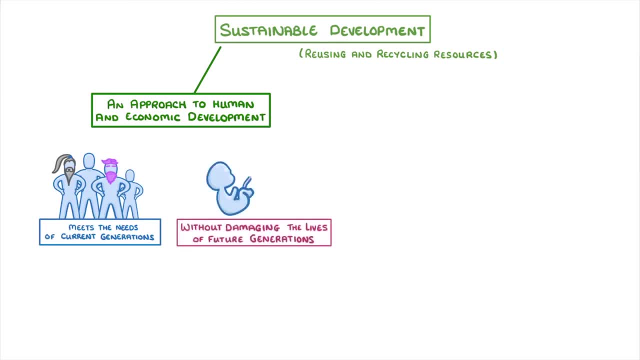 also that it does so without damaging the lives of future generations that are yet to be born. This might all seem a bit vague, but in practice, it basically means that we shouldn't be doing things like using up all the limited resources on our planet or damaging the environment. 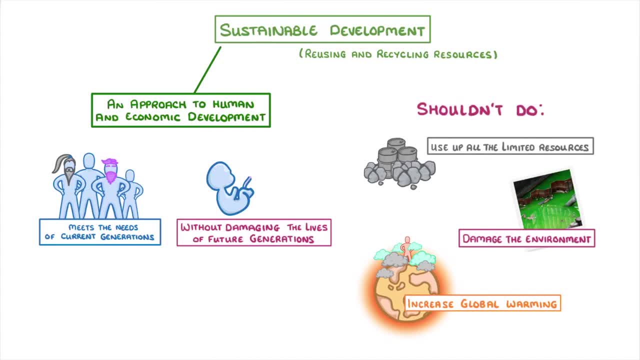 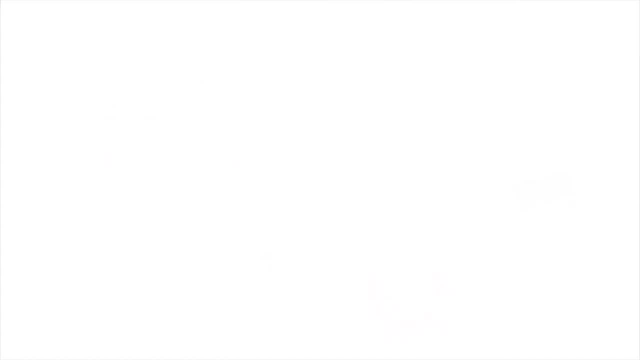 or increasing global warming, because these things will all have negative impacts on future generations. One way that we can develop more sustainably is to use renewable resources rather than finite resources. For example, making products out of wood may be more sustainable than making. 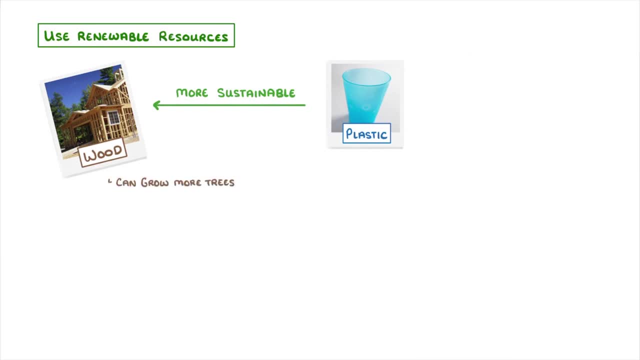 them out of plastic because we can grow more trees, whereas plastic has to come from crude oil, which is a finite resource. Another important thing to take into account is the amount of energy used in the manufacturing process. For example, if making things out of wood is a very important resource, then 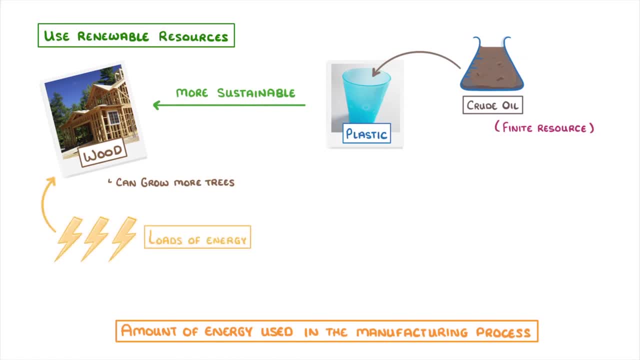 it's important to take into account the amount of energy used in the manufacturing process. If making things out of wood required loads of energy, which we had to get from burning fossil fuels, then it wouldn't really be all that sustainable. Luckily, chemists have come up with ways to reduce the environmental impact of manufacturing. 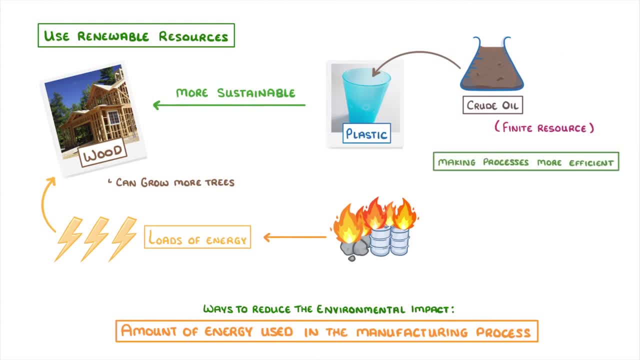 things: either by making processes more efficient- like only needing a tiny amount of oil to make a whole plastic cup- or by reducing the energy required for the process, which they can do by using catalysts, And that's what we're going to do. 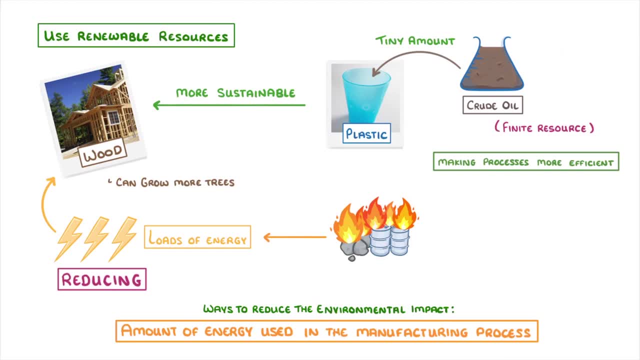 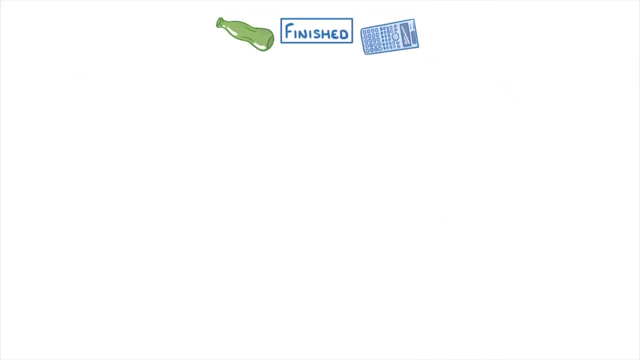 Once we've finished with a product, the most sustainable thing that we can do is to reuse or recycle it. Reusing an item just means to use it again, and that could be for the same purpose or a different purpose. For example, when we're finished with a glass bottle, we 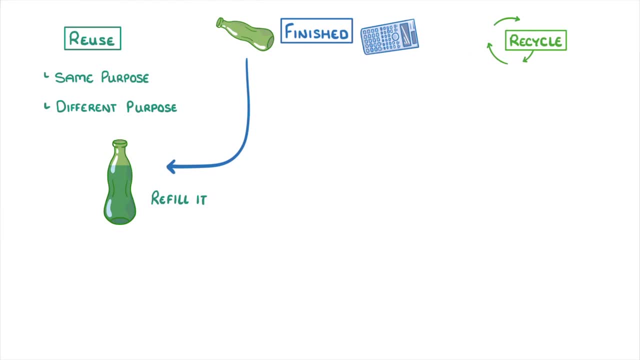